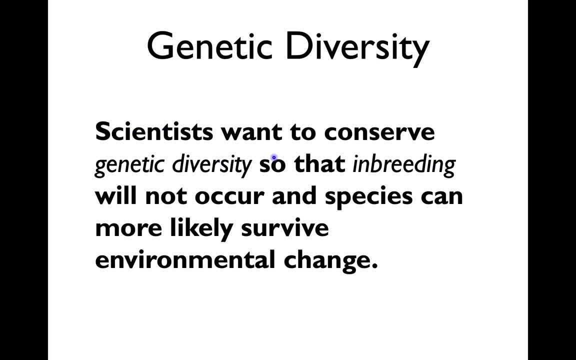 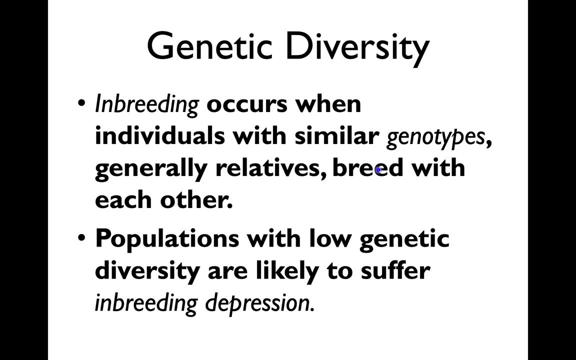 We want to conserve Genetic diversity, because if there's only a small pool of genetic species, they have to breed with each other and then inbreeding can occur. So inbreeding is not a healthy thing for any species. So inbreeding is basically when you have a similar genetic basis, or we call them genotypes. 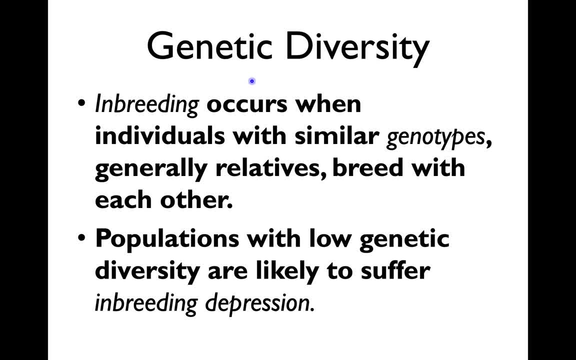 If you breed like if they're relatives to each other, for example. this is what we call inbreeding. So you and your relatives have very similar genetic genotypes And if you would breed with a relative, you would have a higher probability of passing on two sets of bad traits to your, to your children. 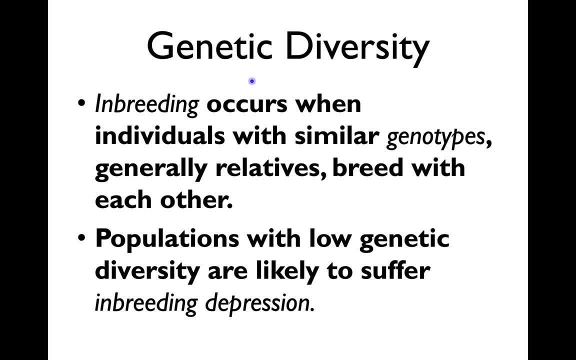 You don't want that, because then they are going to pass those on, et cetera, And you start amplifying these bad genetic traits. So call this. the population with low genetic diversity usually suffer something called inbreeding depression, where inbreeding itself causes the species to not likely to survive. 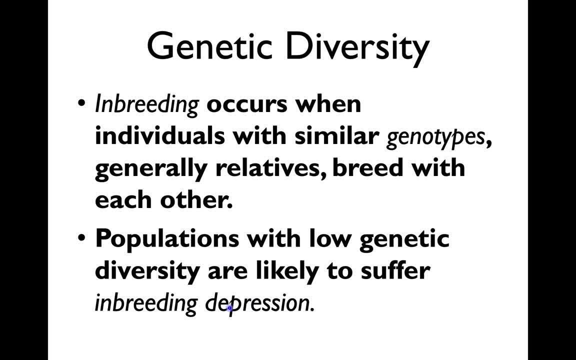 They get bad Genetic traits that cause them to die sooner. So you have this depression of the species population just through inbreeding. So to avoid inbreeding. you want to keep the biodiversity high. You want a lot of different species with different genotypes. 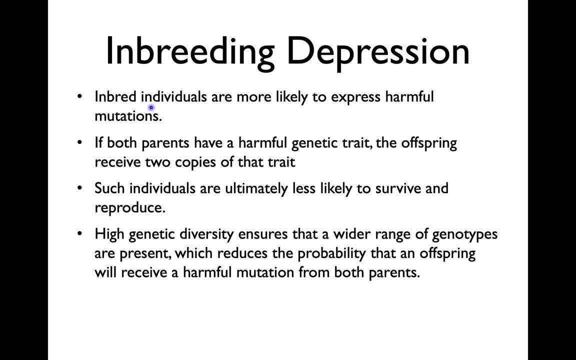 So let's talk about this a little bit more. I added a few more points here. So inbred individuals are more likely to express harmful genetic mutations or genetic traits. So again, if both parents have some really harmful genetic trait, well, their offspring is going to receive two. 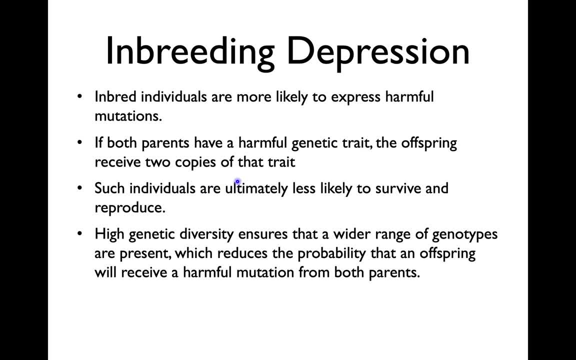 Two copies of that trait. So those individuals are going to be less likely to survive because now they have two of those copies of that trait in their genetic pool. So you want parents that have diverse genetic backgrounds mating with each other, ideally to keep the gene pool more diverse. 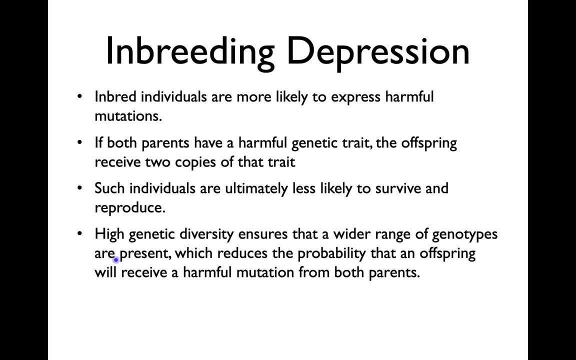 So high genetic diversity ensures that a wider range are present and that that'll reduce the probability that that offspring will receive too harmful Mutations from parents. if they receive one, it might not be that that bad. Maybe the harmful mutation actually is, is not even going to be a problem. 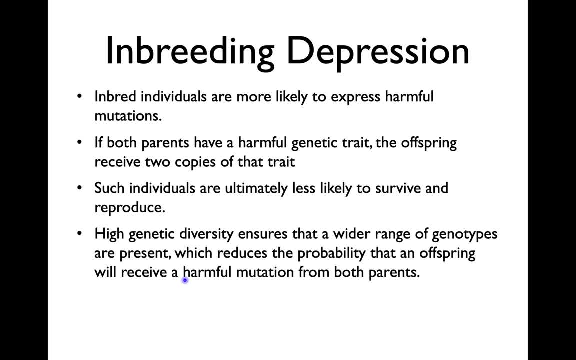 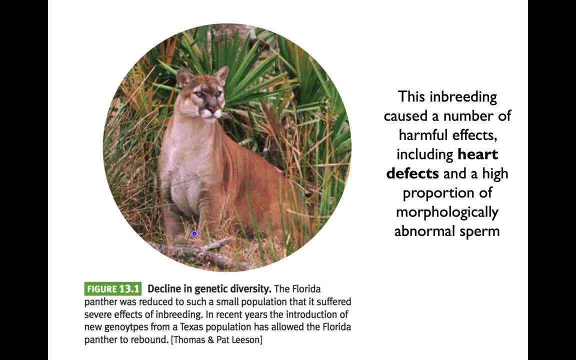 So inbreeding depression is a big issue once you start chopping down the amount of species in the environment And we've seen some specific cases of that over the years. This is one case the book brings up. So there's a species of of panther, the Florida panther, and that kind of cougar type variety. 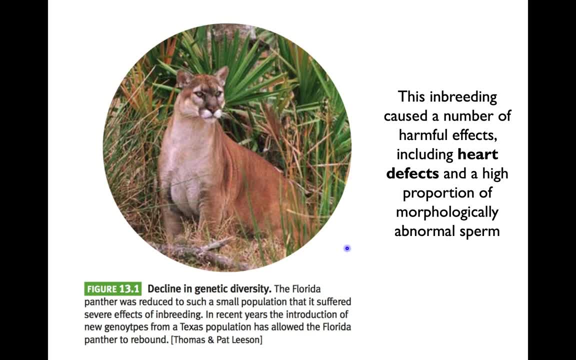 And Due to declining in population, declines in population. these are both natural and anthropogenic human cost. So, for example, there's natural predators like alligators for these type of panthers, but also losing their population, losing their environment through the spread of humans in their area. their population starts to decline. 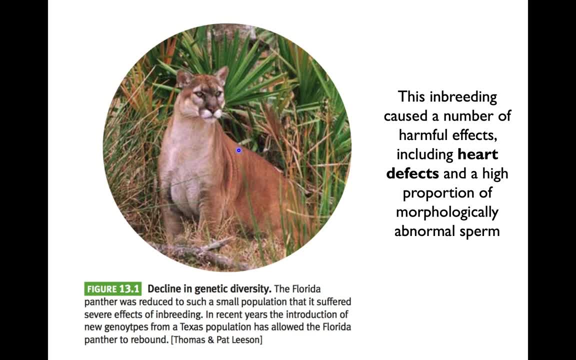 And then what happens is inbreeding occurs. So they have this inbreeding depression effect where they were passing along things like heart defects and Abnormal sperm morphologies, things that decreased the chance of survival for their offspring. So you have this, you have this depression of their populations. 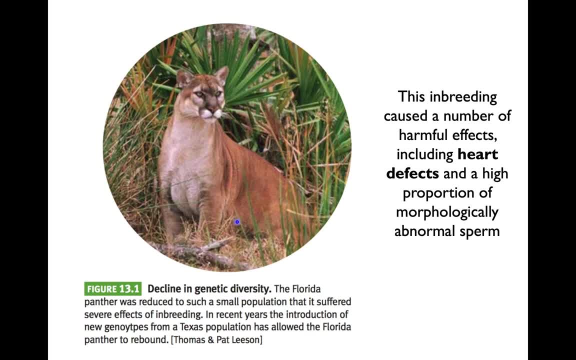 So what they try to do is to increase the diversity of their genotypes. What they did was introduced some Texas population of panthers, so you would add in another population and other species to help breed and increase the biodiversity, And they've seen a bounce back of population of the Florida panther because of this. 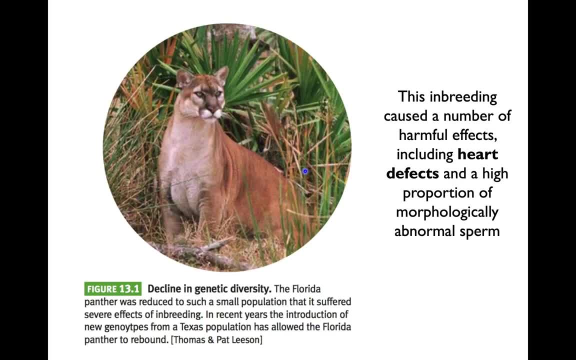 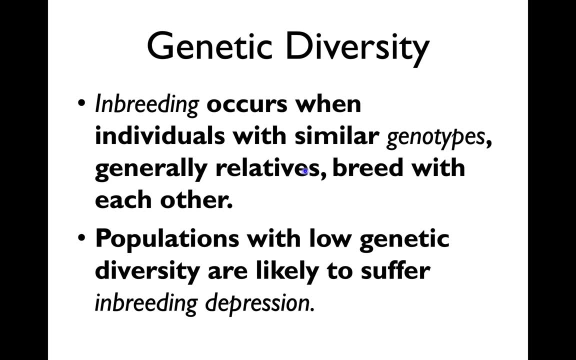 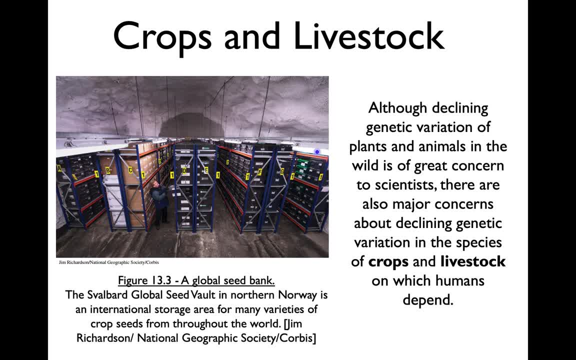 But the other side of this is also crops and livestock, so not wild animals, First of all, crops and the livestock that we actually grow. Trying to keep these genetically diverse is also very important, And it's something that a lot of scientists spend a lot of time thinking about. 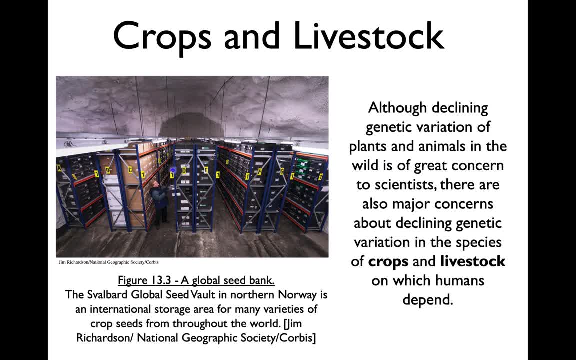 And one of the first things you see in this book is showing you this global seed bank. There's a lot of these around the world. This is an international one where people can come and store seed varieties, And this is built into a mountain to protect it from natural disasters, for example, like a nuclear warhead or something, hopefully, but or just global warming in general. 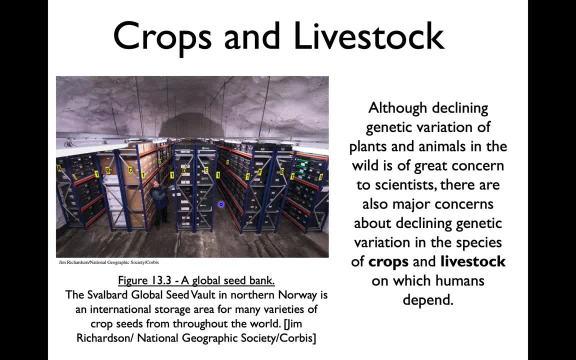 They're kept at a really constant temperature. So there's, there's thousands and thousands of seed varieties stored in here to make sure that we don't lose them, But we don't lose those seeds that we can introduce to the back of the world if we need to. 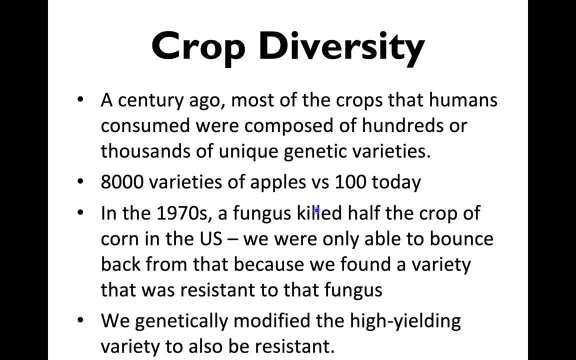 So crop diversity in general, we used to be a lot more diverse in our crops- You would think about all the farmers spread across the country- where they all had their local kind of naturally existing ecosystems, And back then we had a lot more specific and unique ecosystems. 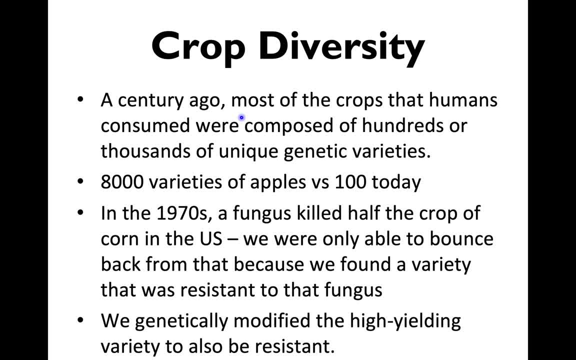 So specific crops would grow at different, specific temperatures and soil compositions, So you'd have all these diverse types of crops. So we used to have thousands and thousands of these varieties, For example, apples. just a century ago we used to have around 8000 varieties of apples versus we kind of are used to seeing about 100, which might seem a lot. 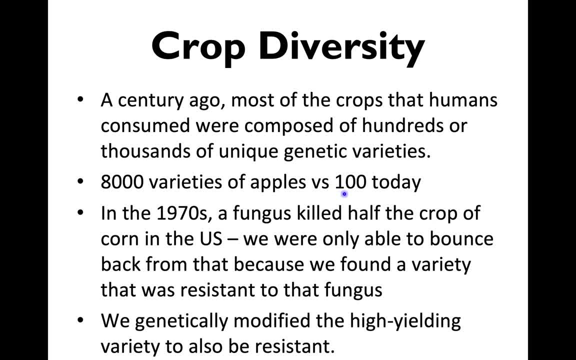 But in the world of genetic diversity that's really small. And then you go to the grocery store and what do you see? You can't even buy 100 varieties of these. You can buy maybe 10 varieties of the grocery store. So we went to 8000 to 100 of just looking at apples. 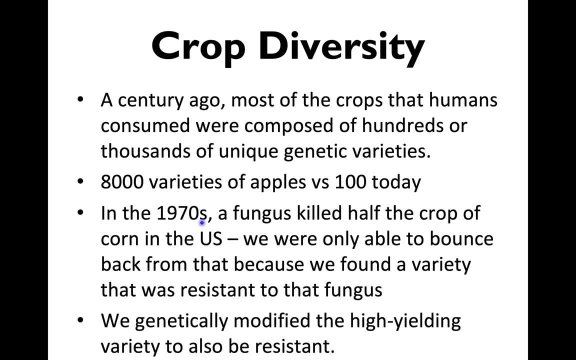 That's just one, One example. So practically what's the problem here? Well, the book goes into this example. In the 1970s there was this fungus that came and killed half the crops in the US of corn. 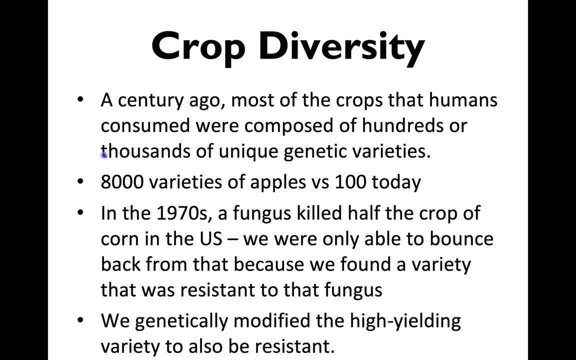 So this corn was selected over the years. That's the problem. here We started noticing which varieties produced a lot high productivity. So we didn't pick for flavor or color or resilience to fungus, for example. We picked for a high productivity. 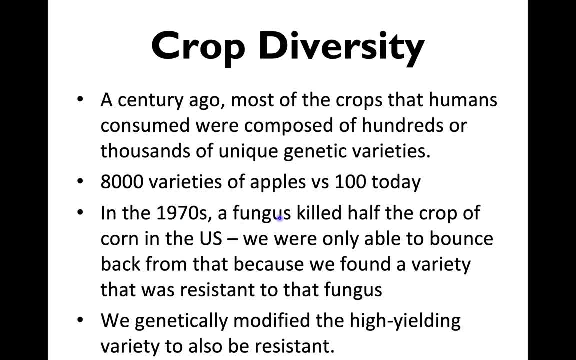 And these high productivity growing corns were not able to combat against this fungus. The only reason we survived this mess is we found another variety of corn that was able to be resistant to this fungus, And we genetically modified the high productivity one to include a gene that was resistant. 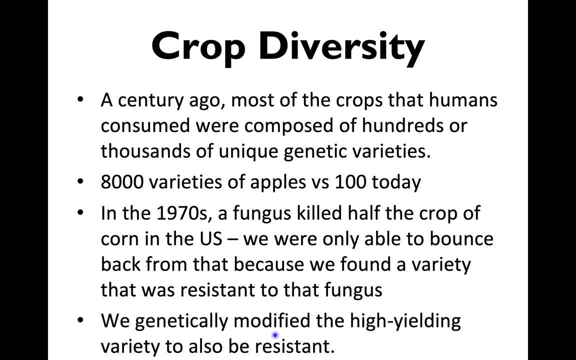 So it was a high yielding variety and also became resistant. If we didn't have that variety, if that other one had died out and got lost, what would we have done? So that's the point: We want to keep as many. We want to have a very diverse, genetically diverse batch of seeds and crops available so that we can combat against these types of issues. 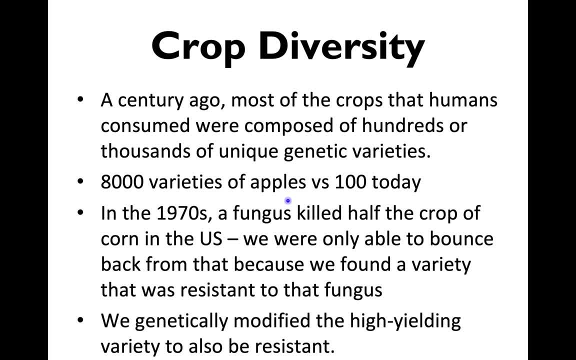 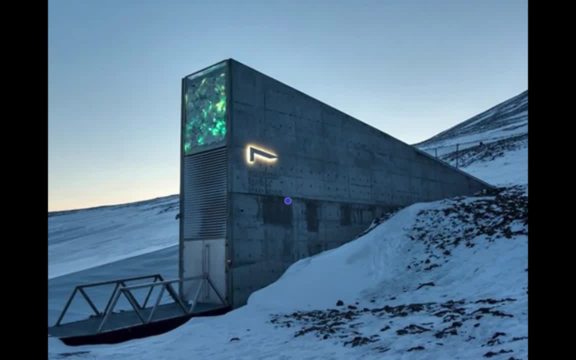 Also, it's just wonderful in the world of culinary cuisine to have more than just the high producing varieties. So this is another picture of that seed ball in Norway. by the way, I found this. There's a lot of these photos. It's pretty striking. 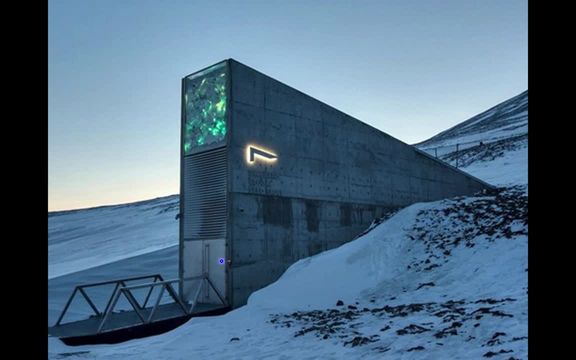 First of all, they took some time in architecture to build a really beautiful, interesting entrance, This kind of a- I don't know, I don't know exactly what is up here- this kind of glass, kind of art piece almost, and this goes directly over the side of this hill, this mountain. 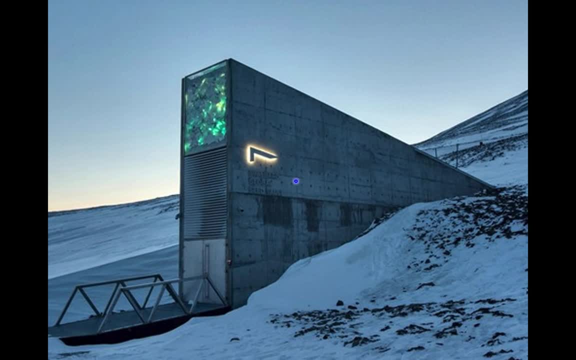 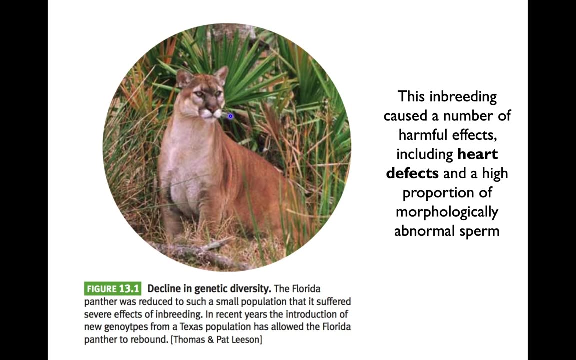 So the seed vault's way down here. This is just a really cool looking entrance. So that's that seed vault in Norway. So yeah, we want to. first of all, you don't want inbreeding to occur. You have that inbreeding depression effect. 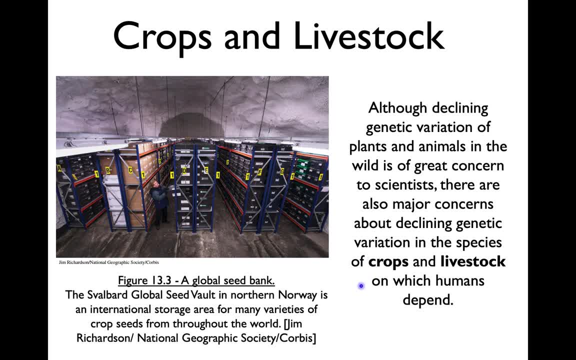 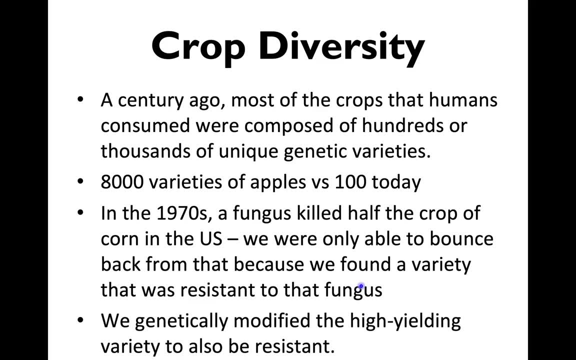 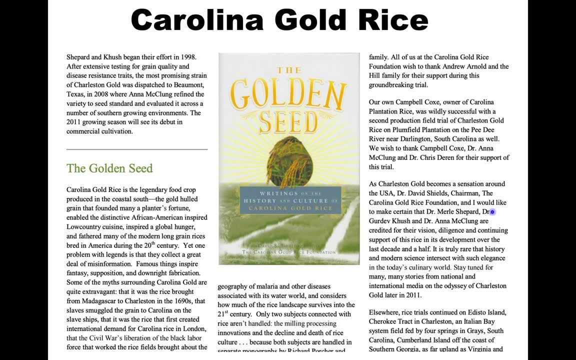 Then for crops and livestock. we want to have healthy variety in the crops and livestock we have. If you think about livestock, Actually, I'll go to livestockcom Just a second. I want to talk about crop diversity In the world of cuisine, for example. I watch a lot of Netflix cooking shows and this Carolina gold rice pops up a lot in some of these shows. 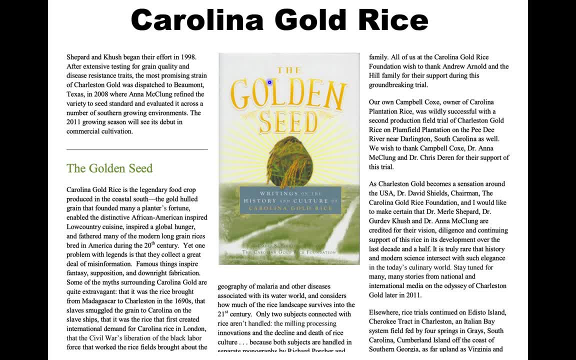 And this is a very renowned and delicious, apparently- rice variety that was almost lost. There's a lot of history in this article about it. It says there's kind of myths of trying to figure out where it came from. Some people think that it was brought from Madagascar in the 1690s. 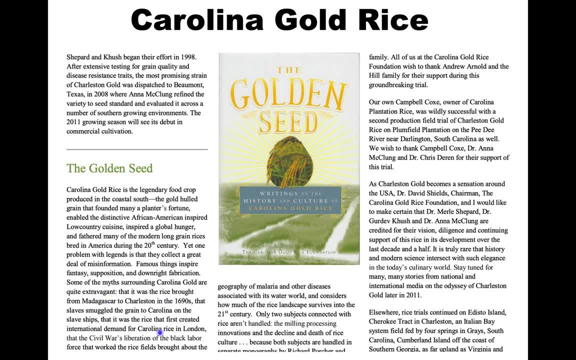 That slaves smuggled the grain to Carolina, That who knows what, But this rice variety was renowned in the South. But, however, as you start selecting for specific types of high-yielding rice, these other ones kind of get lost. But this is a really popular rice now in Southern cuisine and cuisine all over the country. 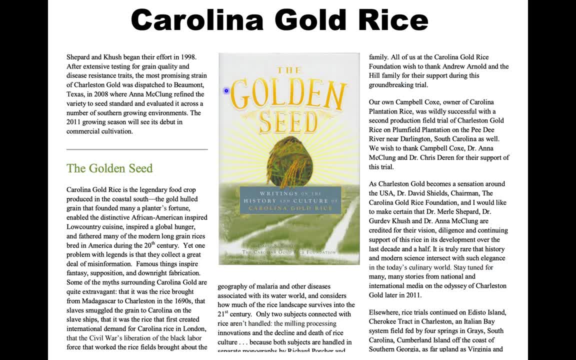 And myself. I would like to order some of this sometime. It's supposed to be just insanely delicious and flavorful And it's just. you know, it's Similar to just normal white rice, but it's a specific variety And we would lose these things unless people went out of their way to save the seeds and cultivate and get these back on the market. 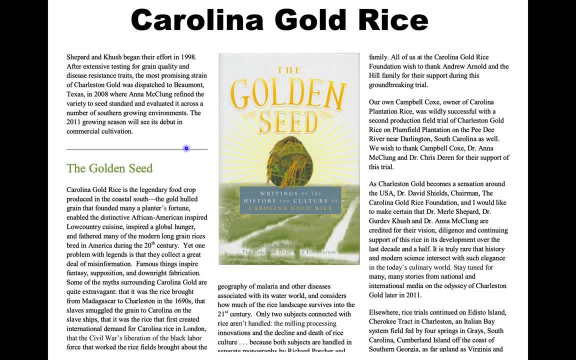 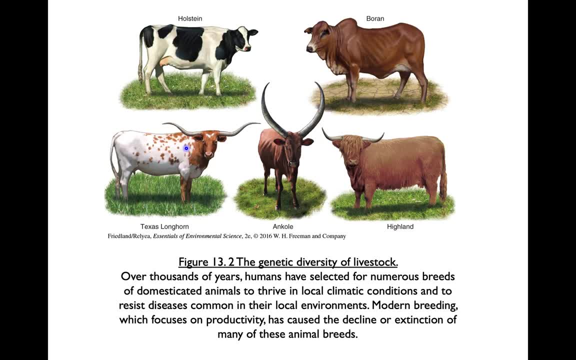 So culinary world, biodiversity of crops. So that's just some other thing I would like to mention. Now livestock: Why do we care about diverse livestock? Well, same kind of reason for the wild animals, If we only select for high. 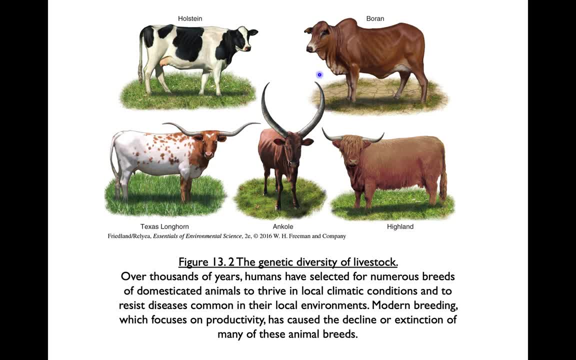 You know, fat or delicious meat or something that we deem ultimately as what we want, we'll lose all the other varieties of these livestock and these lives. We want to. we want a diverse variety, because one livestock might be subjected to a disease, or we want to have the ability to raise livestock that can combat against all different types of effects. 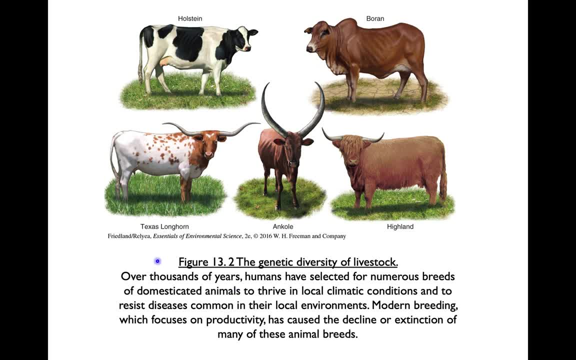 So we want that disease resistant community. So modern breeding, though again focus on high productivity, We start losing out on some of those species that we used to have And we focus more on, you know, the typical ones that we see, like the Holstein one. 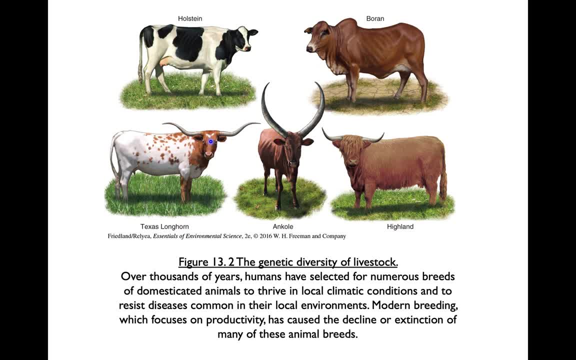 So we've lost a lot of the genetic diversity in livestock over the years as well. So crops, livestock, big deal In terms of the global scene. I wanted to go and actually dig out some more data and kind of think. 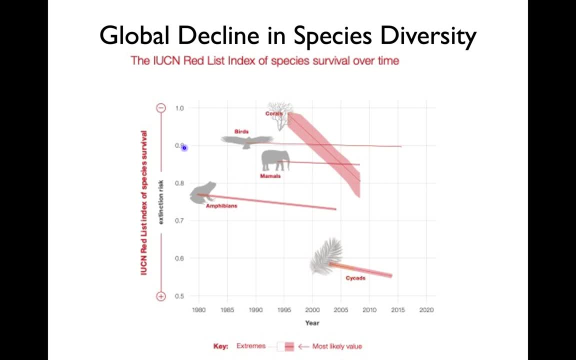 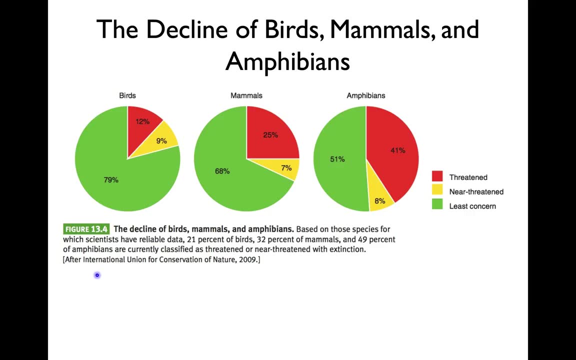 We've only focused on a few different species here, But there's this website of the International Union for Conservation. What is it Actually? let me jump ahead: International Union for Conservation of Nature. There it is. They have lots and lots of data. 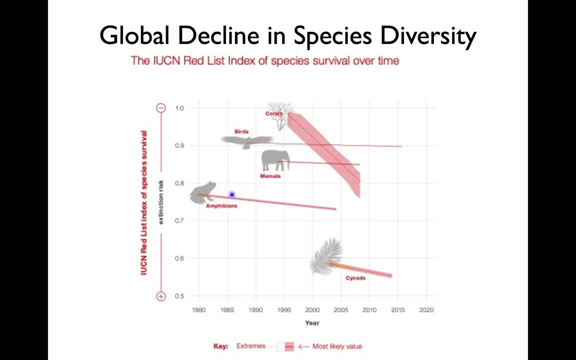 No, this did not turn out. I thought this was going to be a PDF and it is blurry, But bear with me here. on this photo This is from there. They have the so-called red list of index of species And this is their estimation of basically the extinction risk over time for these groups. 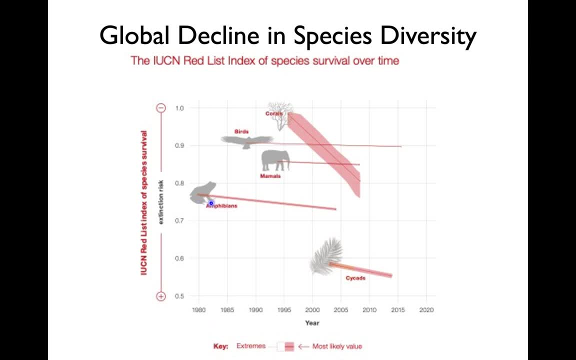 So notice, this starts in the 1980s: Mammals: We've declined a little bit, but we're doing pretty good in terms of their extinction risk In general. I mean this is really broad. Birds have stayed fairly flat, but we also see a decrease. 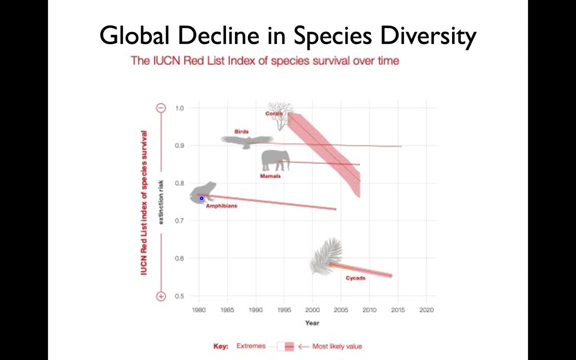 Amphibians have taken a big dive. We are really not doing a great job of keeping the survival risk of the group of amphibians. And look at corals. Corals have just taken a drastic drop in this risk of extinction. A lot of this is due to these bleaching events, where these corals die because of slight differences in temperature or pH in their ecosystems. 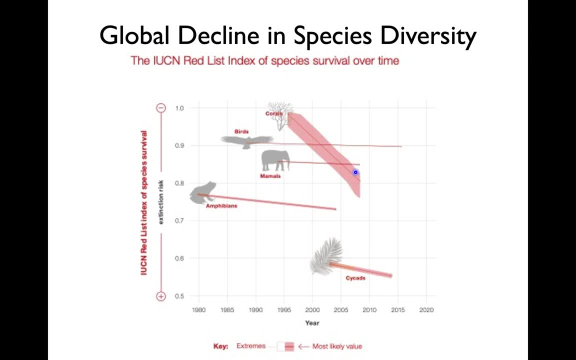 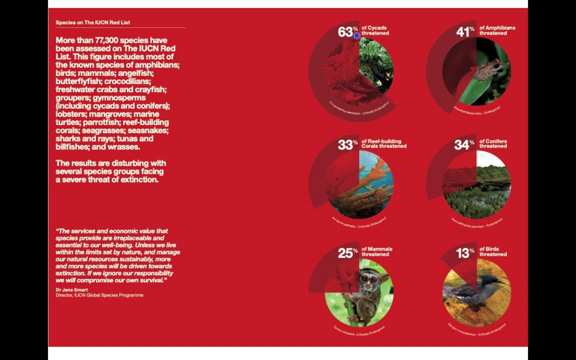 They're very sensitive And we are seeing a really bad dive off of species survival, So we're losing biodiversity because of this extinction risk. Some of the other data that I picked out from this website was on this PDF. Notice again: 41% of amphibians are the threatened variety. Notice birds down here, not so much Mammals- Mammals 25%- but it's these big groups And also these cycads. These are all water-related. So clearly there's a lot going on in the water variety of species where we're seeing a lot of threatened. 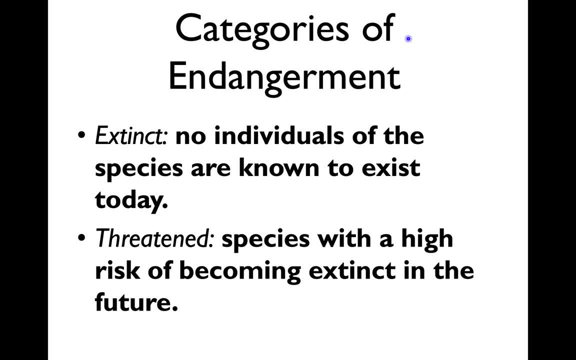 So what do we mean by threatened or endangered? So these are the categories that are generally used to determine the risk level of that species Extinct being. they're gone, So there's zero of them anymore. Threatened is even worse. 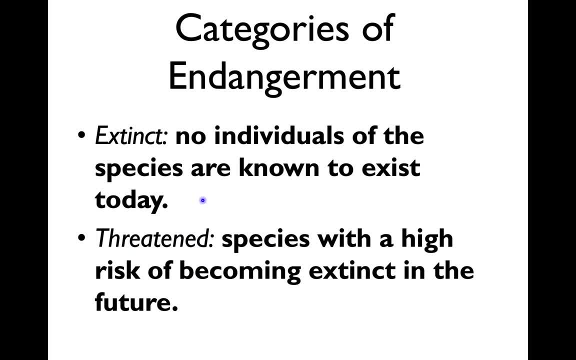 They're worse than endangered. Threatened is there's a high risk of being extinct. So threatened species versus near threatened, for example, and then least concern. These are only four categories. These are broken down into more granular categories as well. 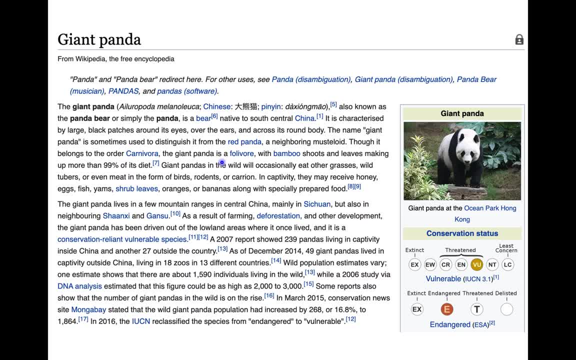 For example, I went to the Wikipedia page for the giant panda. If you ever go to Wikipedia and look up animals on the right-hand side, right away you'll see their conservation status. So notice we've got the broad ESA or the IUCN. 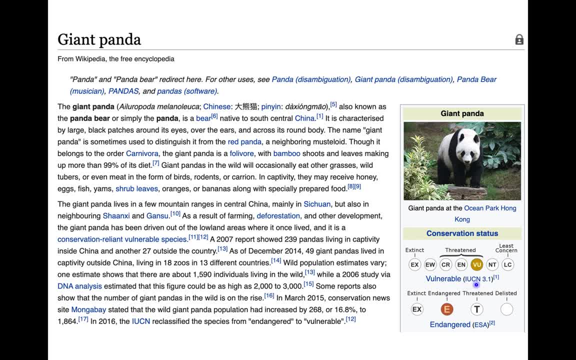 So that's that same group: the International Union And for conservation of nature. this is where these terms endangered and threatened- and the granular ones come in. The ESA uses extinct, endangered, threatened or delisted. They're not on there at all. 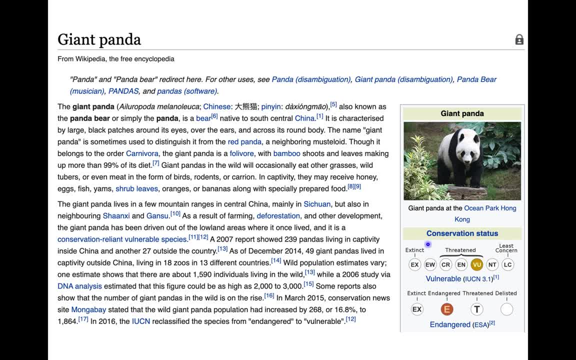 So the IUCN, if you notice extinct, Then EW. I don't actually remember what EW is, But we have endangered, is right there in the middle, Vulnerable, not threatened over here, and then least concern. So, for example, the giant panda, they would say. 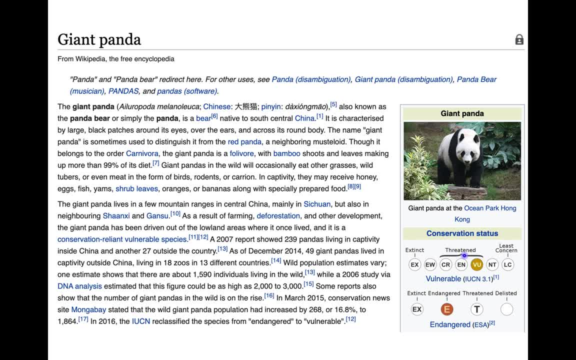 threatened group. all these would be a threatened region to them And vulnerable is on the far end towards almost, almost towards not threatened. So they're not doing too bad. the giant panda. So the book lists some of these, but there are more. 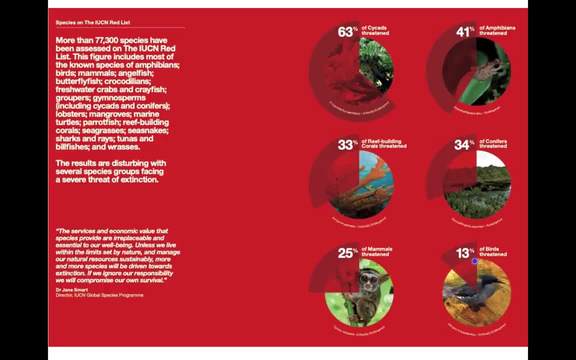 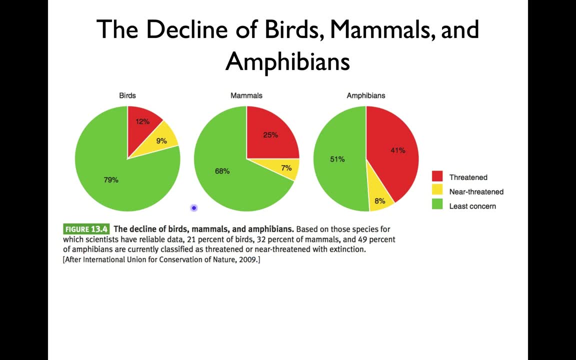 I just want to point that out. And then the book shows this- And this is why I went to this website- because they showed some data from 2009 looking at birds, mammals and amphibians. So if we look at birds, 79% of them are birds. 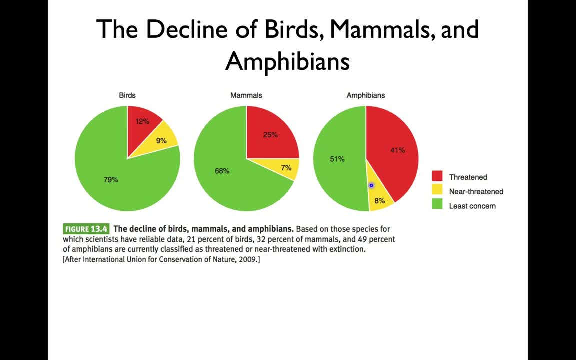 70% of them are in the least concern category, mammals- 68%, but amphibians: only 51% are in the least concern and 41% of them are threatened. So we're seeing a big issue with amphibians right now, and these are the ones that scientists are most concerned about at the moment.